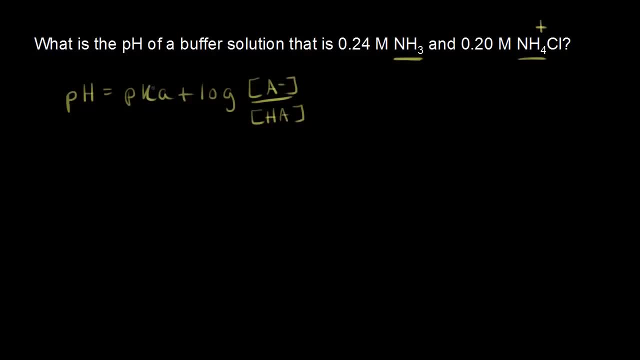 if we're gonna calculate the pH of our buffer solution is to find the pKa, and our acid is NH4 plus. So let's say we already know the Ka value for NH4 plus and that's 5.6 times 10 to the negative 10.. 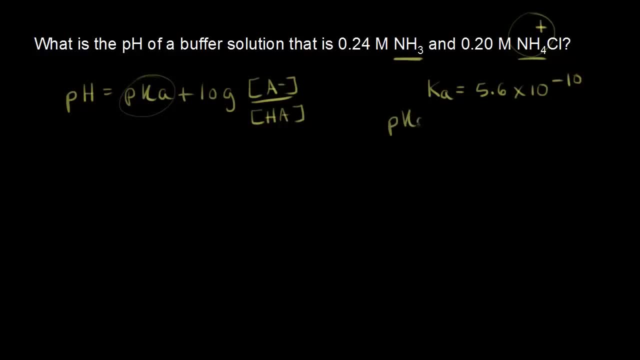 To find the pKa, all we have to do is take the negative log of that. So the pKa is the negative log of 5.6 times 10 to the negative 10.. So let's get out the calculator and let's do that math. 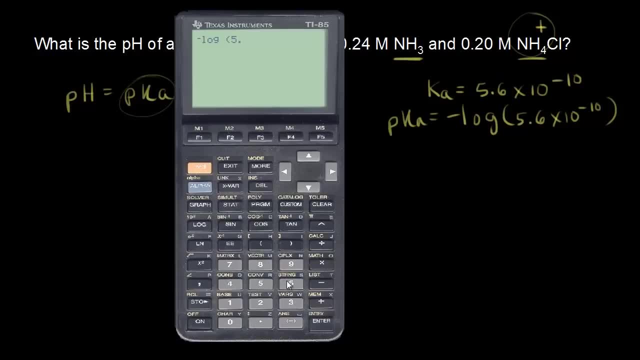 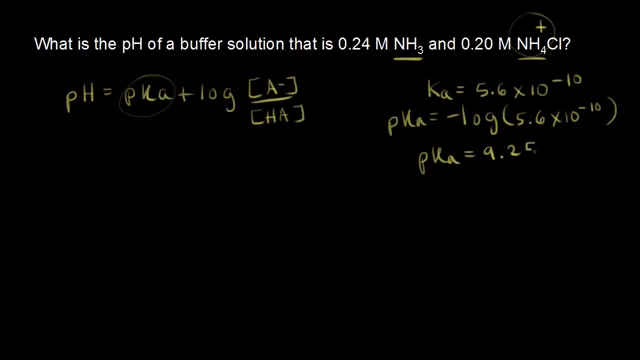 So the negative log of 5.6 times 10 to the negative 10 is going to give us a pKa value of 9.25 when we round So pKa is equal to 9.25.. So we're gonna plug that in to our 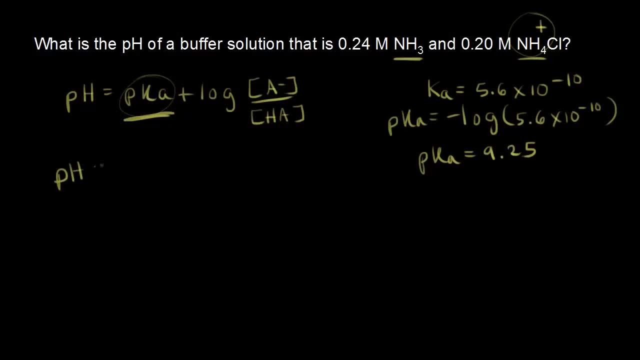 Henderson-Hasselbalch equation right here. So the pH of our buffer solution is equal to 9.25, plus the log of the concentration of A minus our base. Our base is ammonia, NH3, and our concentration in our buffer solution is 0.24 molar. 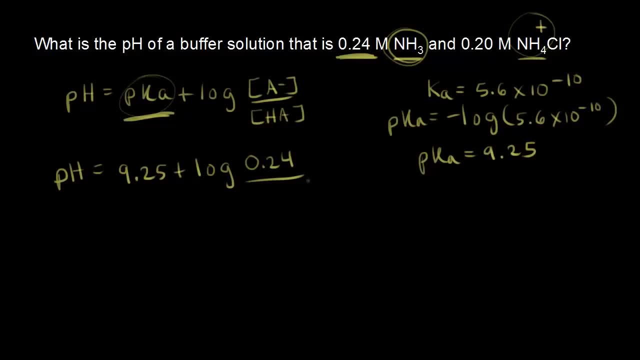 So we're gonna write 0.24 here and that's over the concentration of our acid. That's NH4 plus and our concentration is 0.20.. So this is over 0.20 here and we can do the math right. 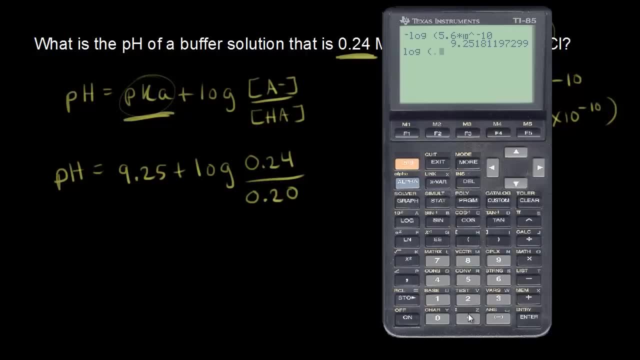 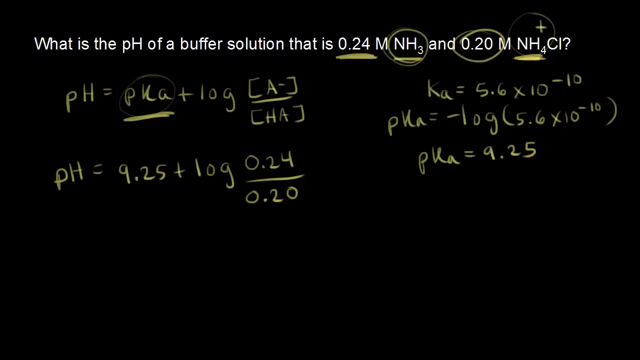 So let's find the log, the log of 0.24 divided by 0.20.. And so that is 0.080, so 9.25 plus 0.08 is 9.33.. So the final pH, or the pH of our buffer solution, is 9.33. 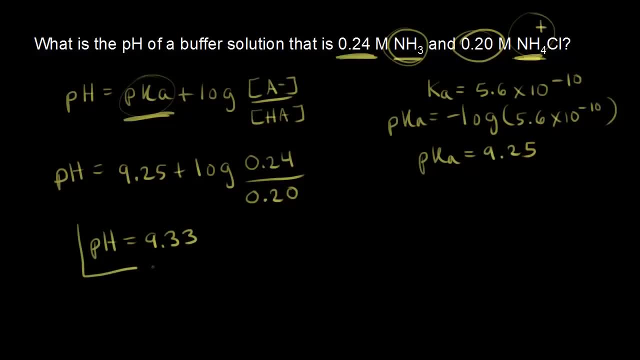 So the final pH, or the pH of our buffer solution, I should say, is equal to 9.33.. So remember this number for the pH, because we're going to compare what happens to the pH when you add some acid and when you add some base. 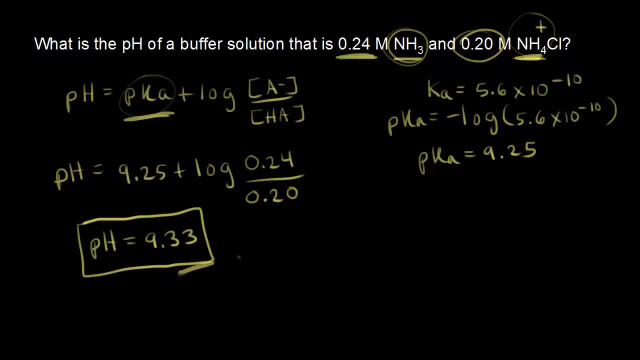 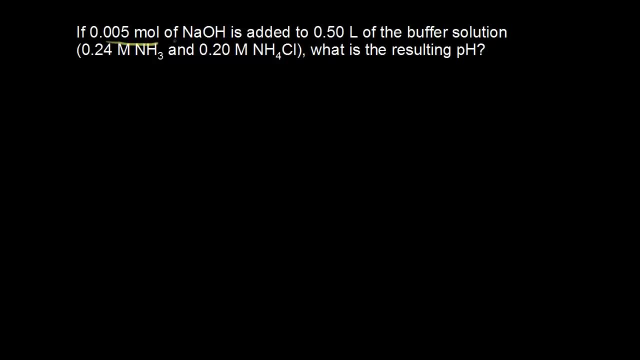 And so our next problem is adding base to our buffer solution, and we're gonna see what that does to the pH. So now we've added .005 moles of strong base to our buffer solution. Let's say the total volume is .1.. 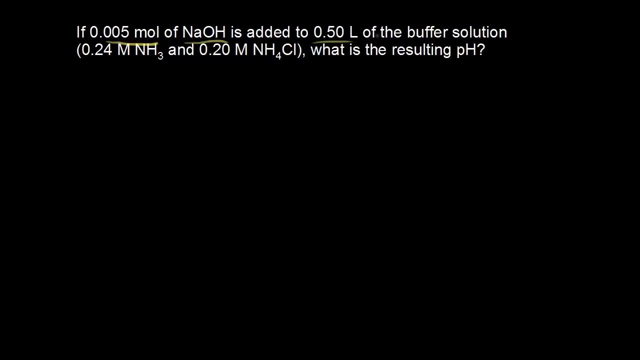 Let's say the total volume is .50 liters. So what is the resulting pH? So we're adding .005 moles of sodium hydroxide and our total volume is .50.. So if we divide moles by liters, that'll give us the concentration of sodium hydroxide. 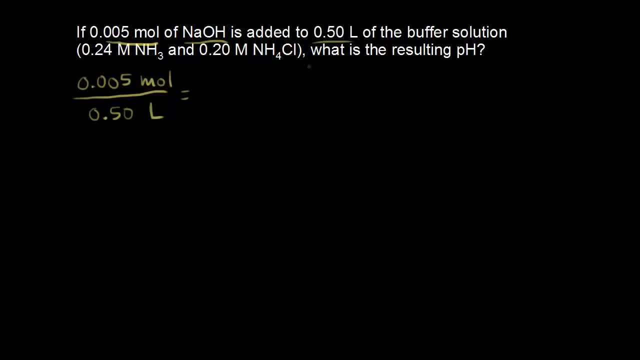 .005 divided by .50 is 0.01. Molar. so that's our concentration of sodium hydroxide, And since sodium hydroxide is a strong base, that's also our concentration of hydroxide ions in solution. so this is our concentration. 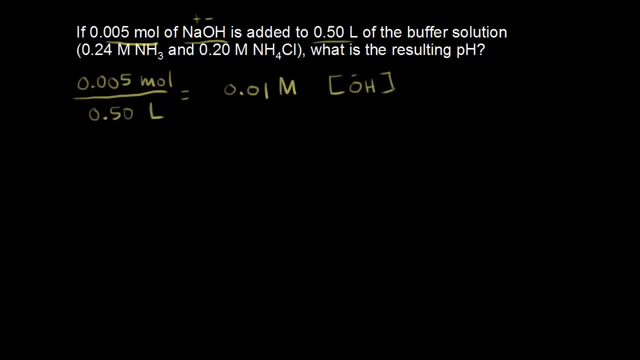 of hydroxide ions .01 molar. So we're adding a base and think about what that's going to react with in our buffer solution. So our buffer solution has NH3 and NH4+. The base is going to react with the acid. 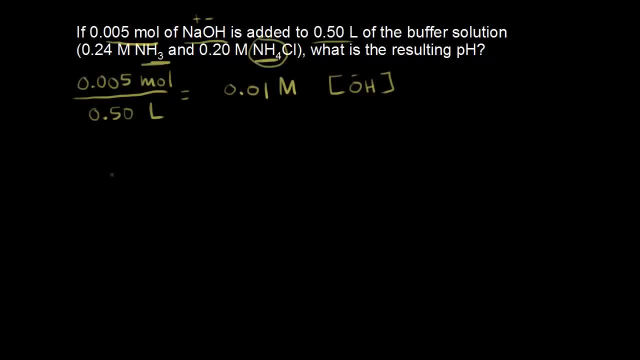 so hydroxide is going to react with it, with NH4+. Let's go ahead and write out the buffer reaction here. So NH4+ ammonium is going to react with hydroxide and this is going to go to completion here. 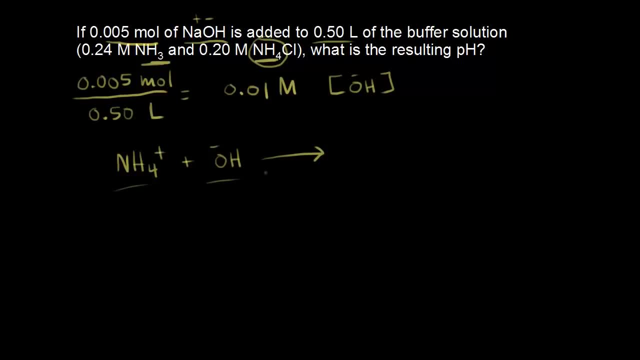 So if NH4 plus donates a proton to OH minus, OH minus turns into H2O, right, So we're gonna make water here, And if NH4 plus donates a proton, we're left with NH3, so ammonia. 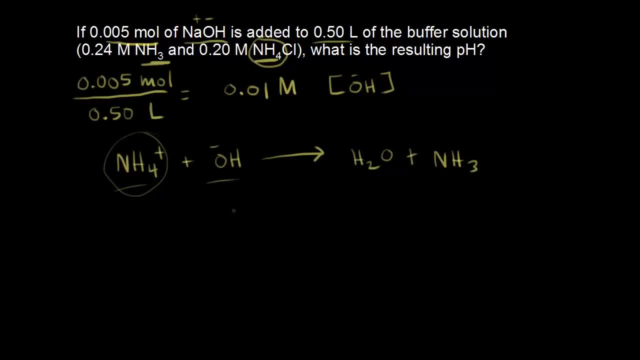 All right, let's think about our concentrations. So we just calculated that we have now .01 molar concentration of sodium hydroxide For ammonium, right, that would be .20 molar. So 0.20 molar for our concentration. 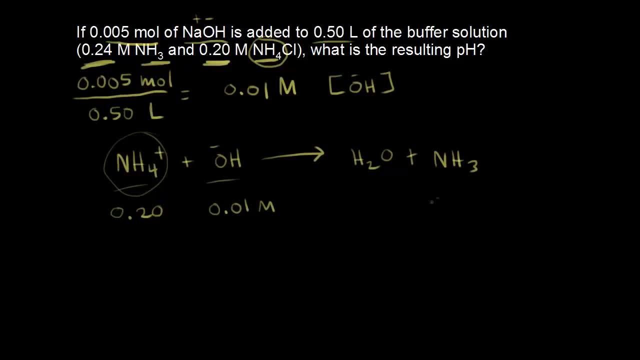 And for ammonia it was .24.. So let's go ahead and write 0.24 over here. So if .01, if we have a concentration of hydroxide ions of .01 molar, all of that is going to react. 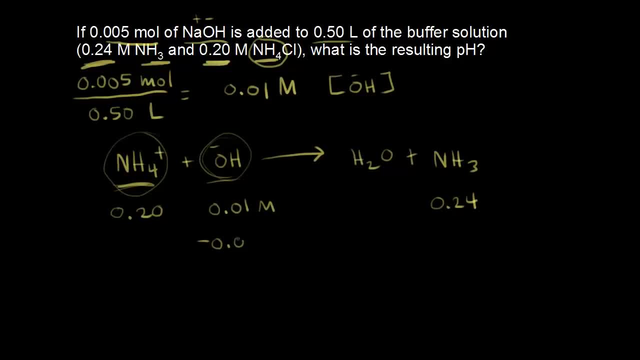 with the ammonium right. So we're gonna lose all of this concentration here for hydroxide and that's going to neutralize the same amount of ammonium over here. So we're gonna be left with right. this would give us 0.19 molar. 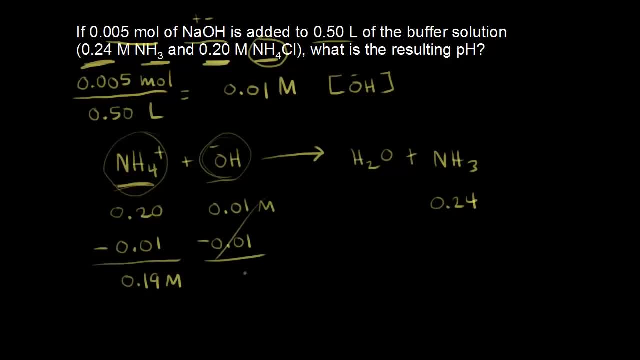 for our final concentration of ammonium right Hydroxide. we would have zero after it all reacts. And then the ammonium, since the ammonium turns into the ammonia right. if we lose this much, we're going to gain the same concentration of ammonia. 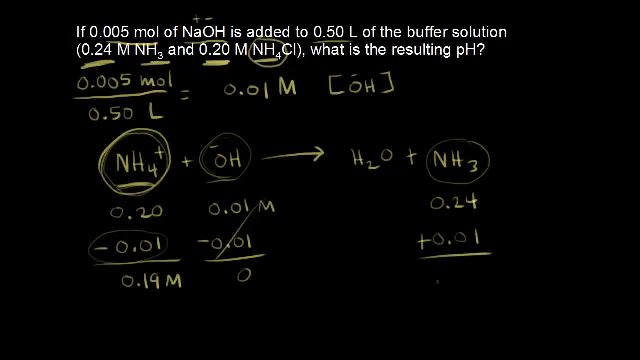 So over here we put plus 0.01.. So the final concentration of ammonia would be 0.25 molar. And now we can use our Henderson-Hasselbalch equation, right. so let's go ahead and plug everything in. 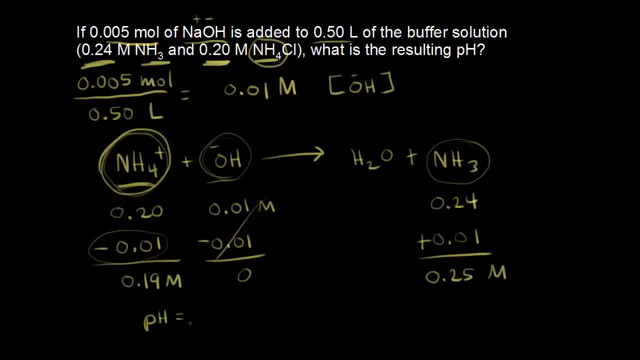 So pH is equal to the pKa. We already calculated the pKa to be 9.25.. And then plus, plus the log of the concentration of base, right, so that would be NH3, so the concentration of 0.25.. 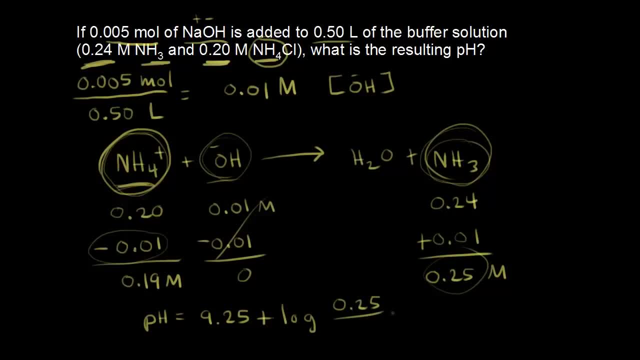 So this is 0.25 molar for our concentration over the concentration of our acid right, And that's ammonium, so that's over 0.19.. So this is all over 0.19 here. So if we do that math, let's go ahead. 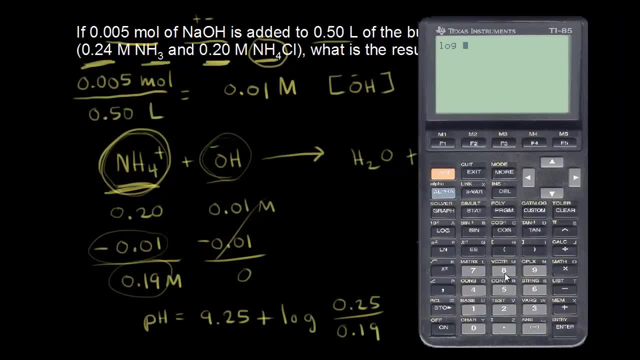 and get out the calculator here and let's do this calculation Log of 0.25 divided by 0.19 and we get, we get 0.12.. So 9.25 plus 0.12 is equal to 9.37, right. 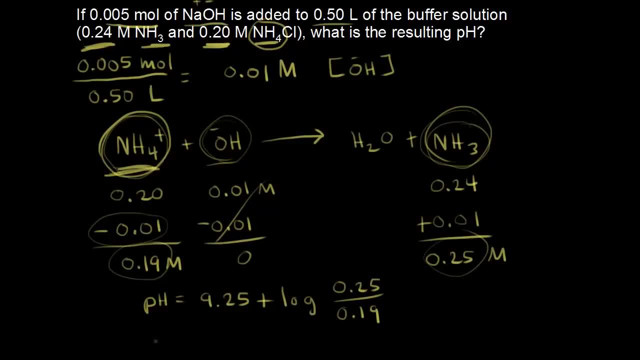 So let's get a little bit more room down here and we're done. The pH is equal to 9.25 plus 0.12, which is equal to 9.37.. So let's compare that. So let's compare that to the pH we got. 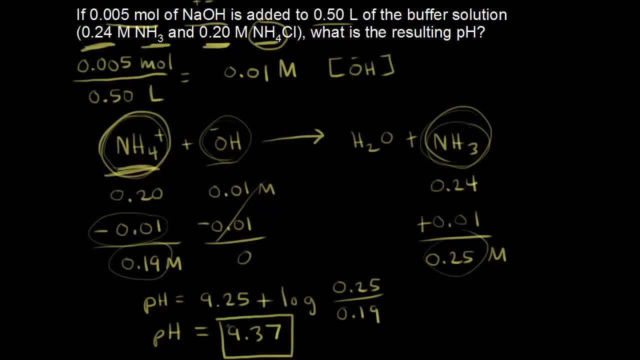 in the previous problem, right For the buffer solution. just starting out, it was 9.33.. So we added a base and the pH went up a little bit, but a very, very small amount. So this shows you mathematically how a buffer solution. 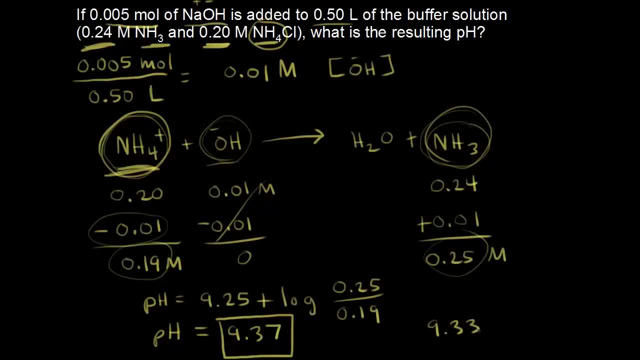 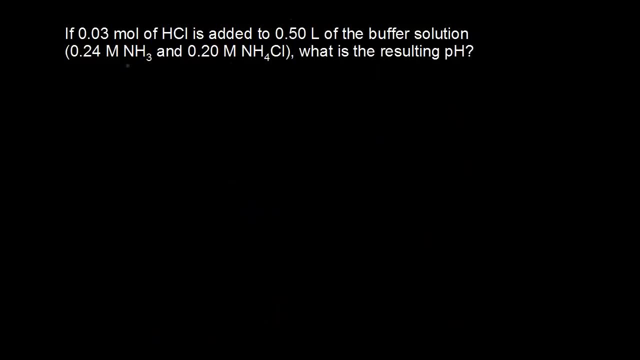 resists drastic changes in the pH. Next, we're gonna look at what happens when you add some acid. So we're still dealing with our same buffer solution with ammonia and ammonium NH4 plus, But this time instead of adding base. 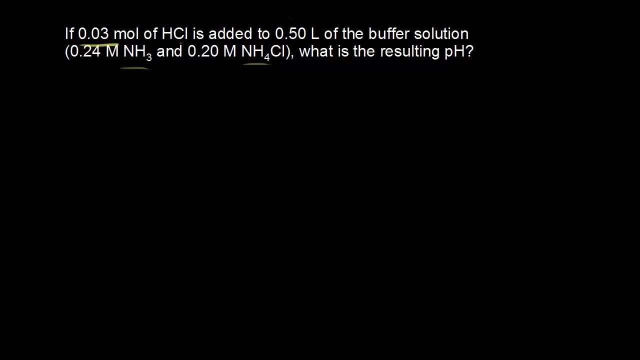 we're gonna add acid, So we add 0.03 moles of HCl and let's just pretend like the total volume is 0.50 liters And our goal is to calculate the pH of the final solution here. So the first thing we could do is calculate. 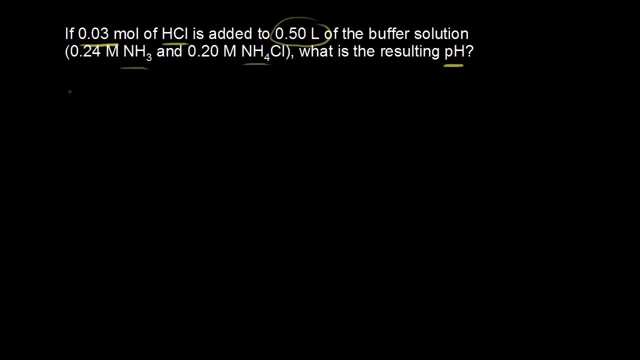 the concentration of HCl right. So that would be moles over liters. So that's 0.03 moles divided by our total volume of 0.50 liters, and 0.03 divided by 0.5 gives us 0.06 molar right. 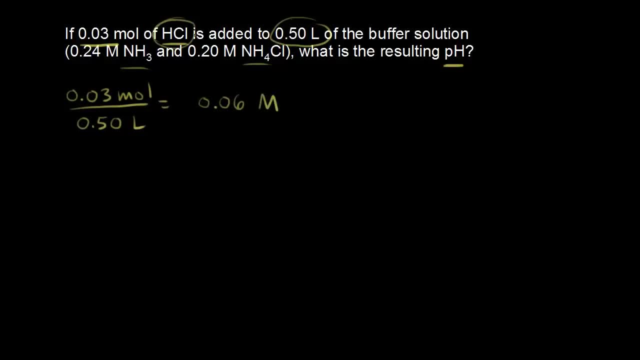 That's our concentration of HCl, And HCl's a strong acid, so you could think about it as being H plus and Cl minus, And since this is all in water, H plus and H2O would give you H3O plus or hydronium. 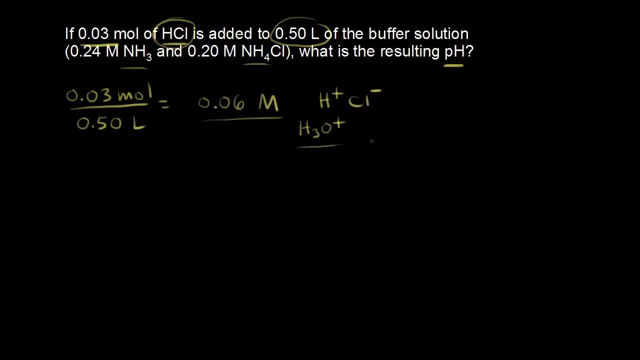 So 0.06 molar is really the same amount of HCl, So 0.06 moles is the concentration of HCl. So 0.06 moles is really the concentration of hydronium ions in solution, And so the acid that we add is going to react. 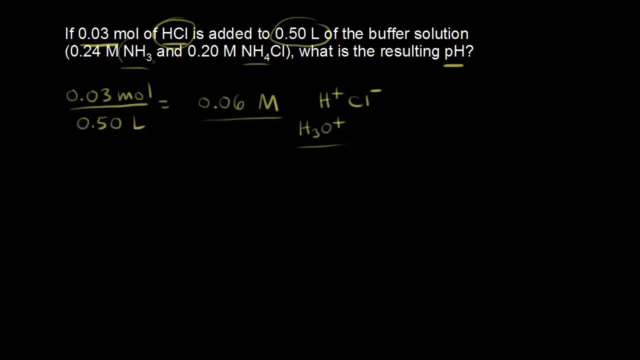 with the base that's present in our buffer solution. So this time our base is going to react, and our base is, of course, ammonia. So let's write out the reaction between ammonia, NH3, and then we have hydronium ions in solution, H3O plus. 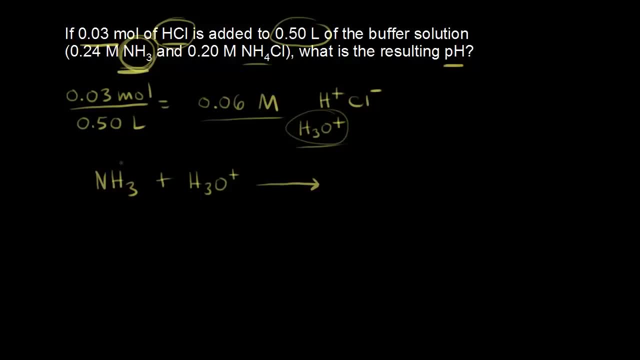 All right. so this reaction goes to completion, And if ammonia picks up a proton, it turns into ammonium And H4 plus, And if H3O plus donates a proton, we're left with H2O. So we write H2O over here. 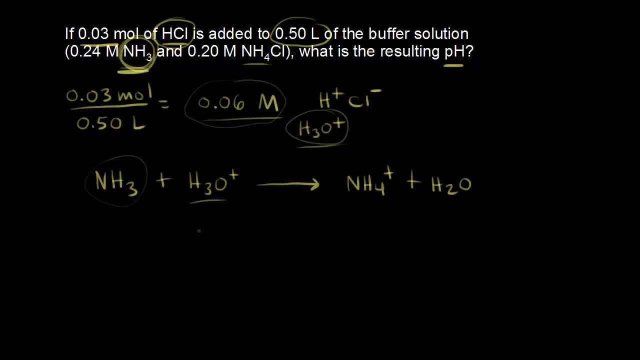 All right for our concentrations. we're going to have 0.06 molar for our concentration of hydronium ions, so 0.06 molar And the concentration of ammonia is 0.24, to start out with. 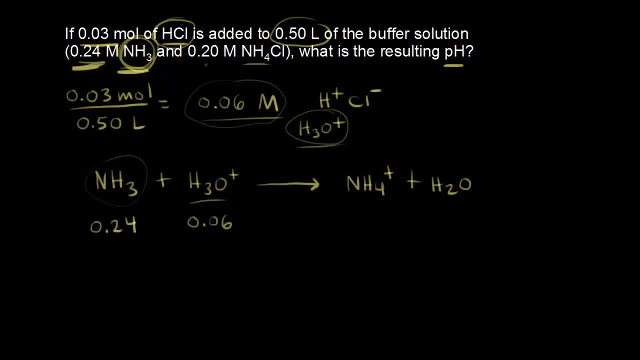 So we have 0.24.. And for ammonium it's 0.20.. So we write 0.20 here. So all of the hydronium ion is going to react, So we're going to lose all of it. 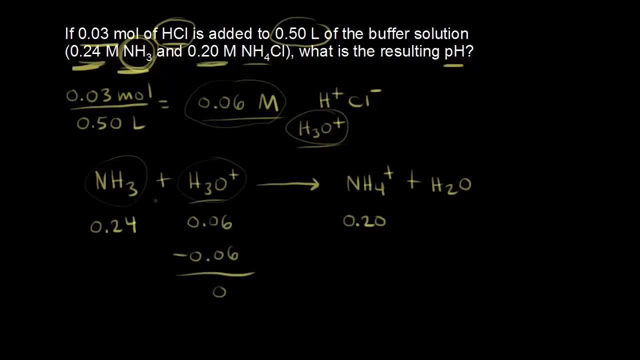 So we're left with nothing after it all reacts. So it's the same thing for ammonia. So we're going to lose the exact same concentration of ammonia here, So we're going to lose 0.06 molar of ammonia because this is reacting with H3O plus. 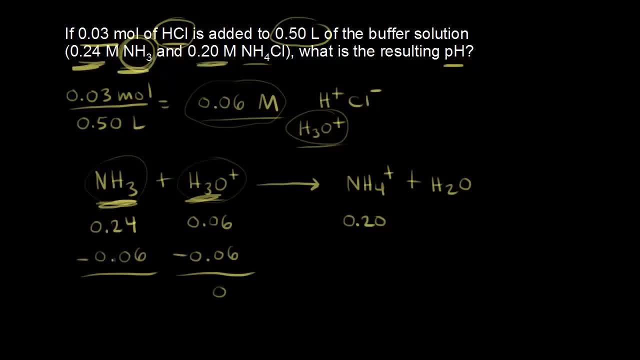 And so, after neutralization, we're left with 0.18 molar for the concentration of ammonia, And whatever we lose for ammonia, we gain for ammonium, since ammonia turns into ammonium. So we're going to gain 0.06 molar for our concentration. 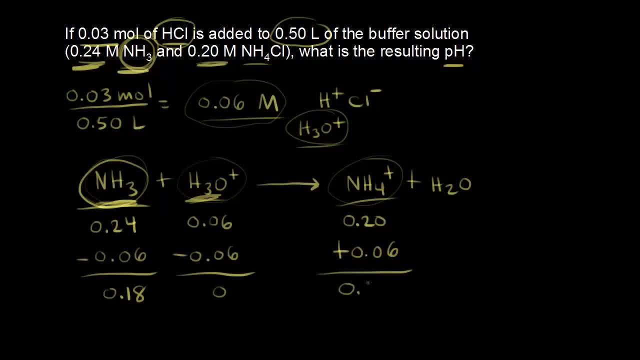 of ammonium after neutralization. So we get 0.26 for our concentration, And now we're ready to use the Henderson-Hasselbalch equation to calculate the final pH. So let's do that, All right, get some more space down here. 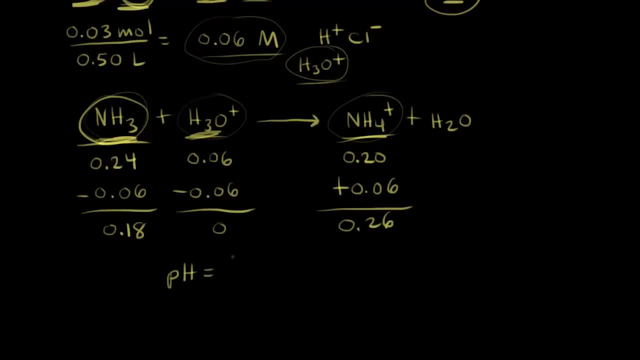 So the pH is equal to the pKa which again, we've already calculated in the first problem- is 9.25 plus the log of the concentration of the base, and that's 0.18.. So we put 0.18 here divided by the concentration. 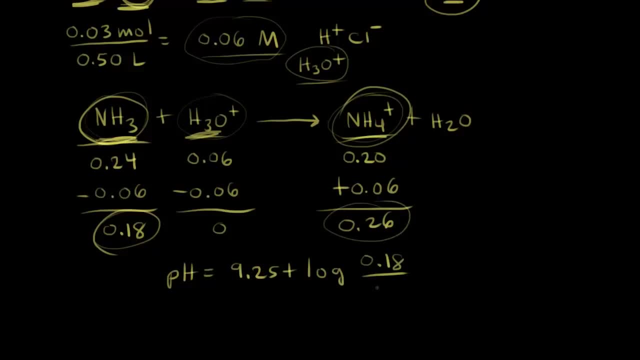 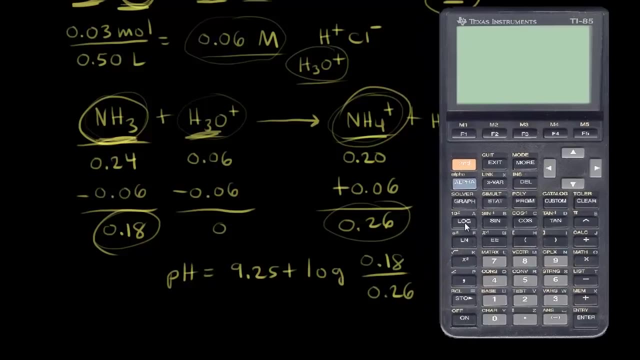 of the acid, which is NH4 plus, So that's 0.26.. And we go ahead and take out the calculator and we plug that in. So log of 0.18 divided by 0.26 is equal to negative 0.16.. 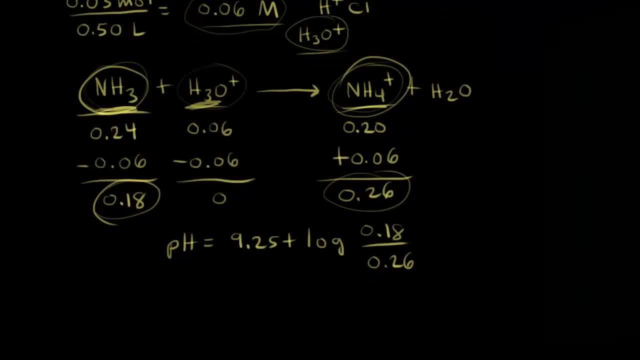 So let's go ahead and write that out here. So we have: our pH is equal to 9.25 minus 0.16.. And so that comes out to 9.09.. So the pH is equal to 9.16.. 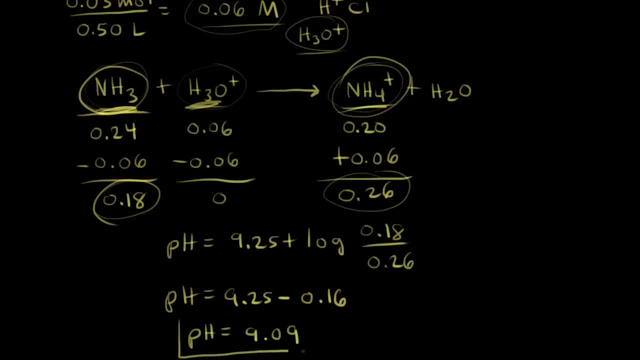 So remember, for our original buffer solution we had a pH of 9.33.. So we added a lot of acid. The pH went down a little bit, but not an extremely large amount. So once again, our buffer solution is able to resist drastic changes in pH.